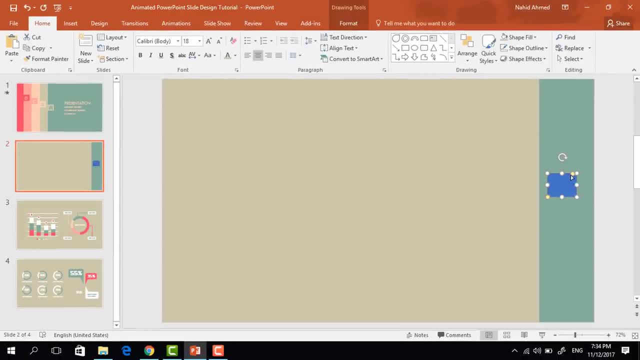 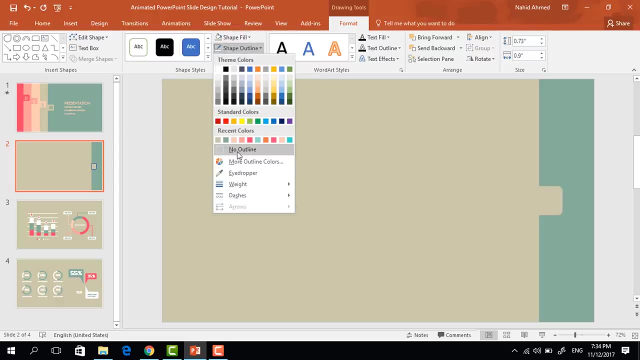 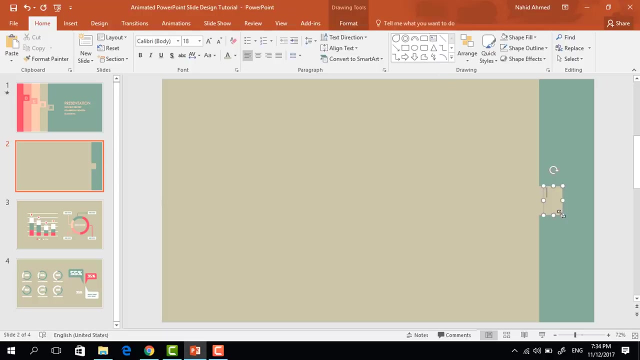 rounded corner rectangle. drag it over here, increase the roundness a bit, rotate it and place it in the exact middle of this rectangle. Now again, change this color and remove the outline. After that, pick a text box, drag it over this small rectangle. Here I'm typing the letter A. select the text, change the. 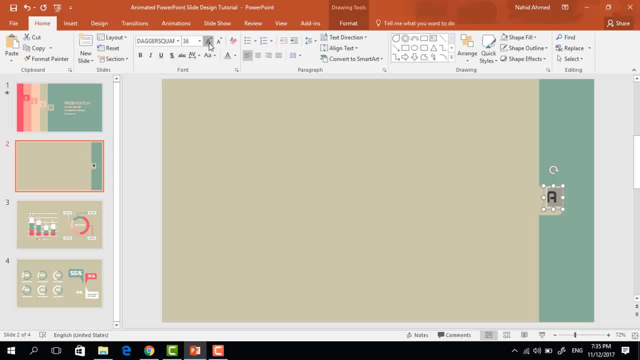 font to dagger square. increase the font size to 48 point. Change the font size to 48 point. Change the font color and make it Center. Now place this text box in the exact middle. Now we need to select these two and press ctrl G to group them together. then press ctrl A to select all of. 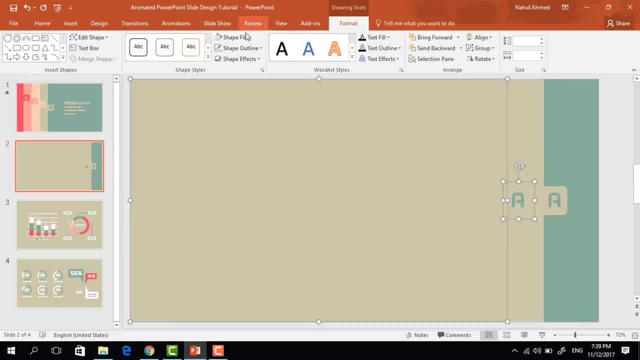 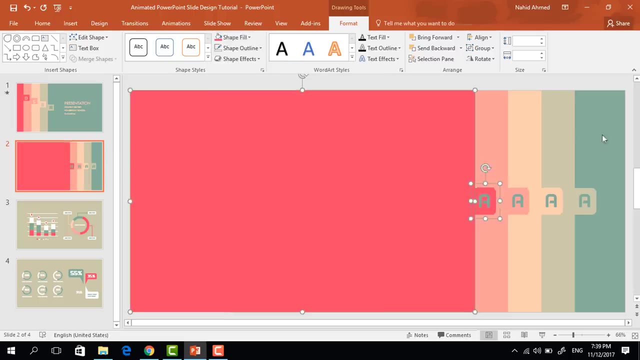 these and, holding ctrl shift, drag it to left. Now change the color from shape fill. again holding ctrl shift, drag it to left. it will be duplicated Again. change this color. i'm doing the same thing for the last time. after doing so, you just need to organize this. 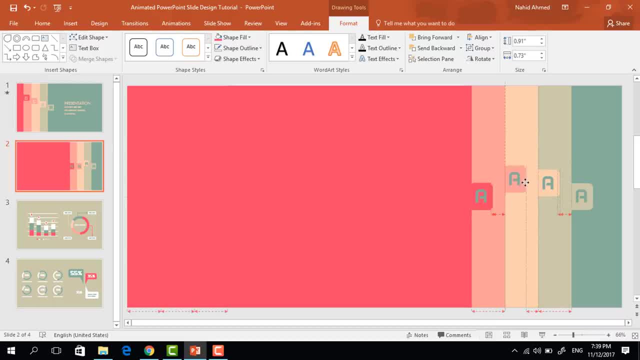 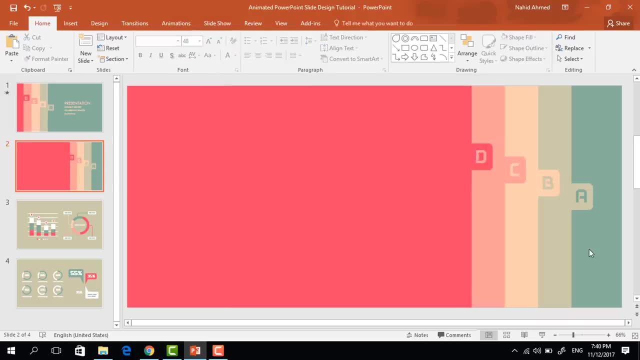 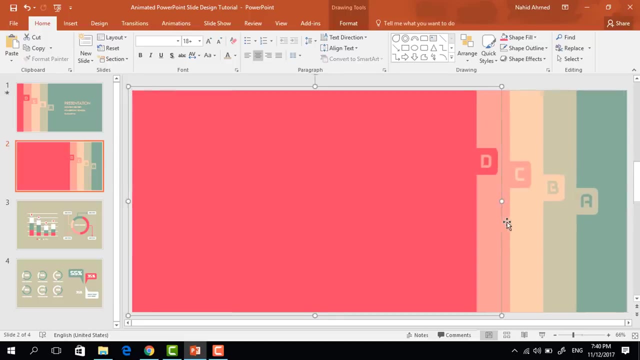 smaller group of shapes- that's why i'm taking them a bit upward- and then change the letter and its color. after changing all the letters, we will have something like this: now we have to group them together one by one. so first, select this two: press ctrl g to group again. select this two press. 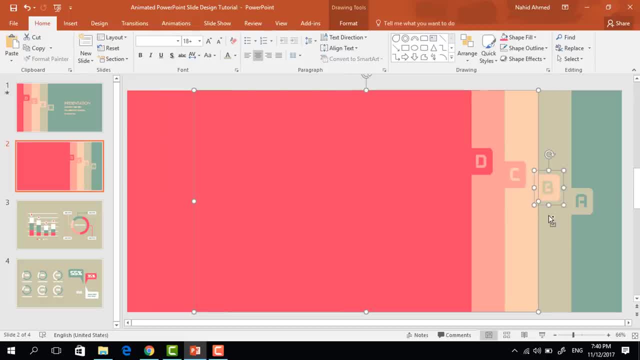 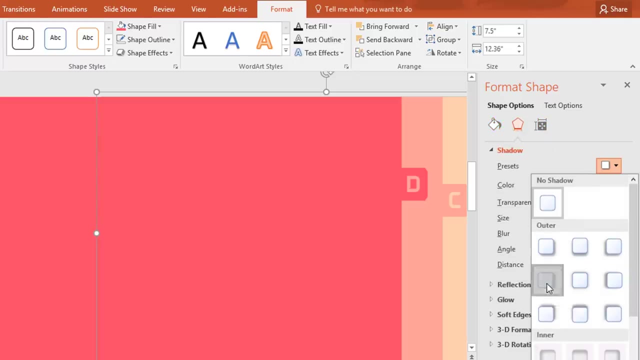 ctrl g to group. do the same for this one and also for this one. so now we have four different group of shapes. from here, select the first one, go to format, click on the small icon, go to effects and set the shadow preset. offset right, change the transparency to 49 percent size, 100 percent blur. 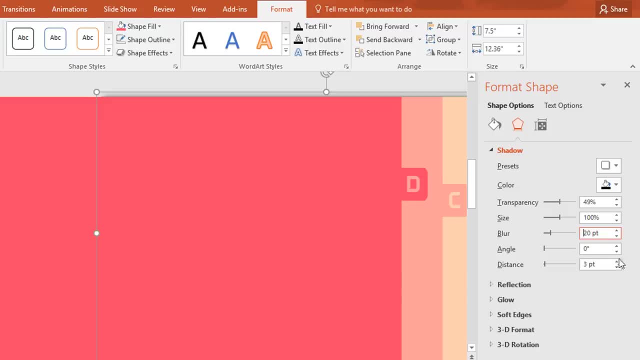 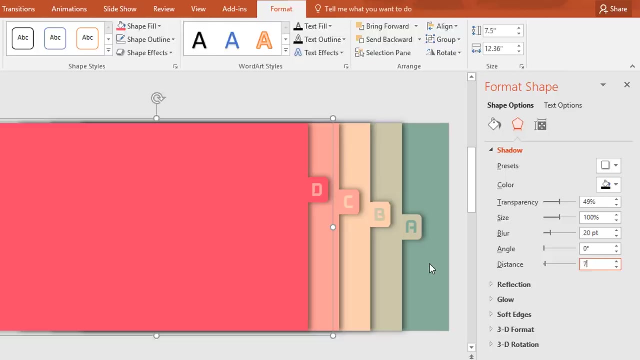 20 point. keep the angle 0 degrees and distance 7 point. here you can see that a shadow has been added on our first element. now select the second one at the same preset. change the transparency to 49 percent. blur: 20 point. distance: 7 point. like this way, we have to add the same shadow on the other elements. 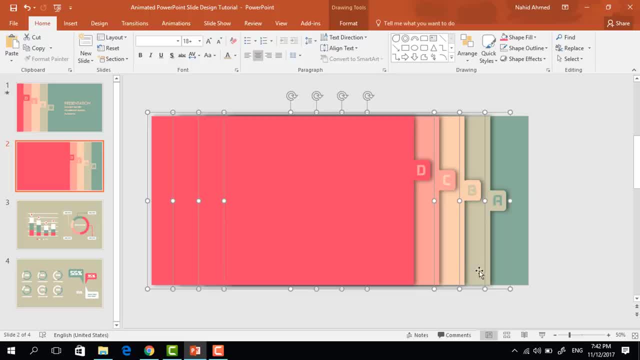 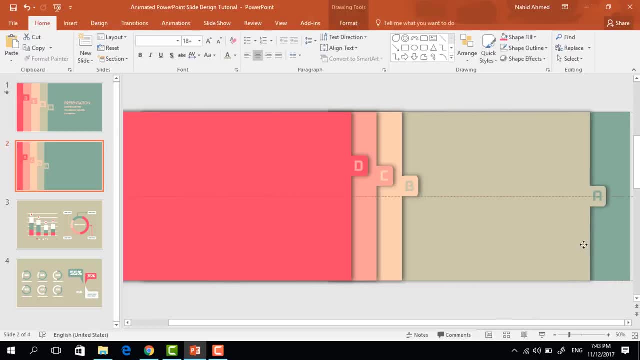 after that, press ctrl a to select all of these and place them to the left side. now, Now, from here, first bring this one to the right side. To save your time in this tutorial, I'm not gonna show you how to make these infographic. 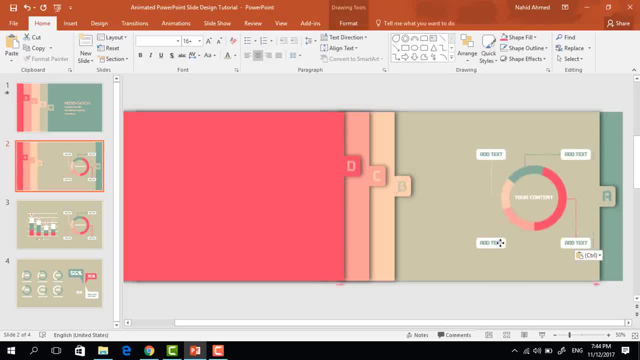 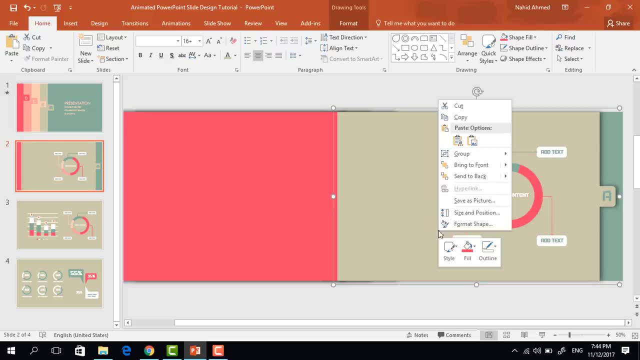 elements. So I'm just copying and pasting them. Place it here holding the ctrl button, select these two and press ctrl g to group, Right click on it and send it to back. Then bring the second one to the right side and from here I'm copying this element and 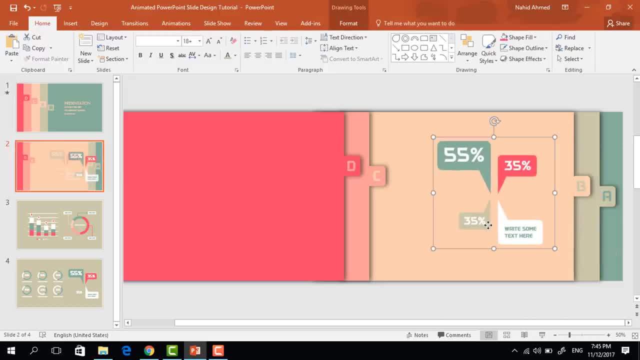 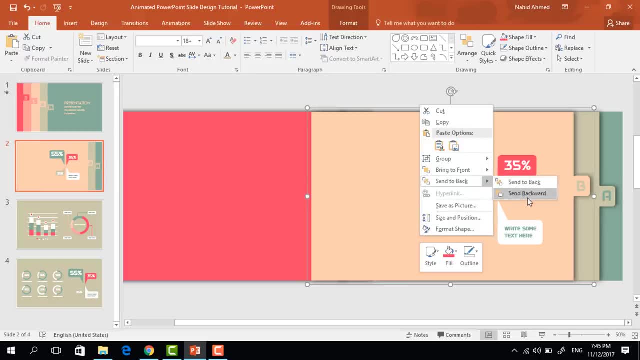 pasting it over here. Now place it here. select these two. press ctrl g to group, right click on it. send it to backward again, right click on it. send it to backward once again. Now bring the third one to the right, copying this chart: 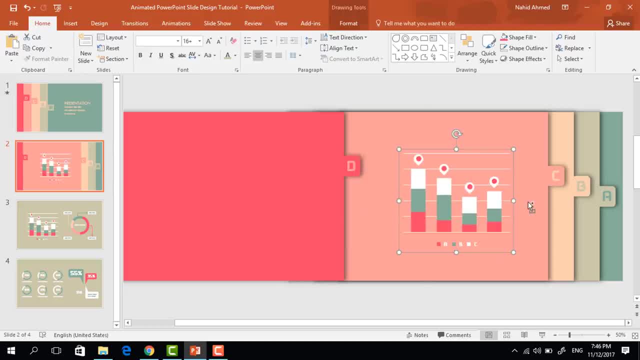 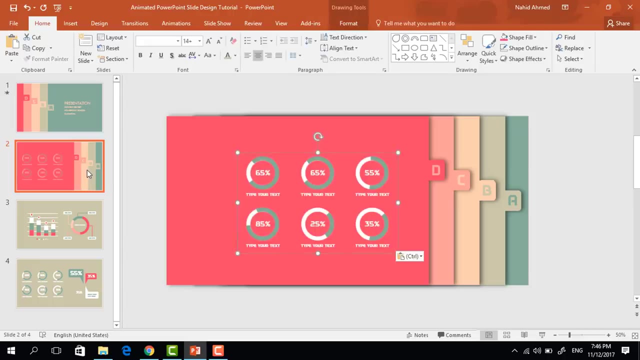 Pasting it over here now. select these two, press ctrl g to group, right click on it and send it to backward For the last time. bring it to here again. copying this element, pasting it over here. select these two and press ctrl g to group. 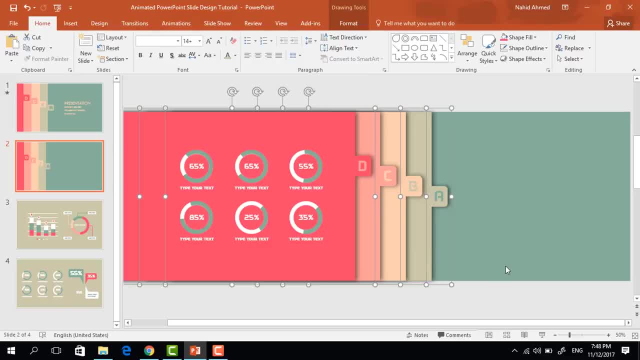 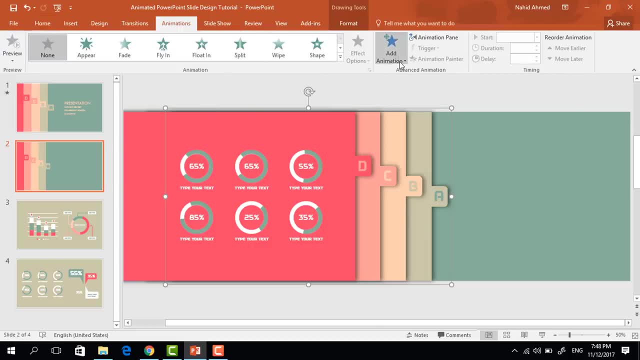 Again. place all of these to the left side, and now we'll add the animation one by one. First, select this one. go to animation. click on add animation from motion path. select lines from effect option. select right. Now drag this red dot to the right. keep it on. click and duration: 1.25 seconds. 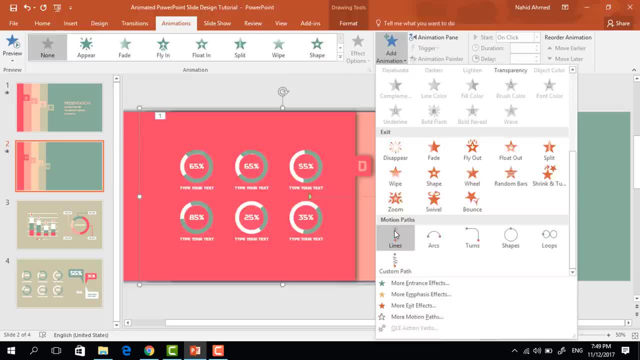 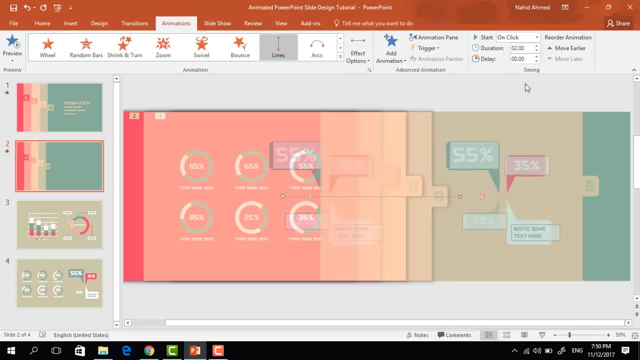 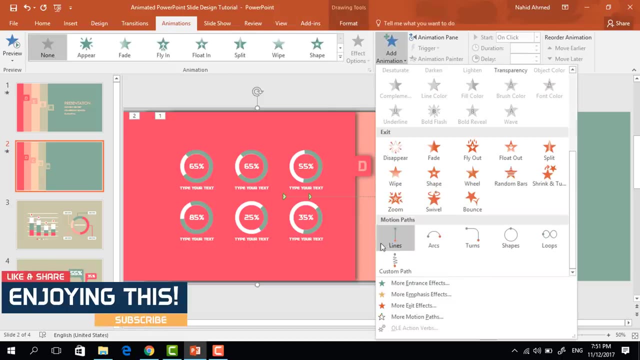 Now select the second one. click on add animation. select lines again from effect option, select right. Drag this red dot again. Set the duration 1.25 seconds. Now select the third one. click on add animation: select lines from effect option, select right.